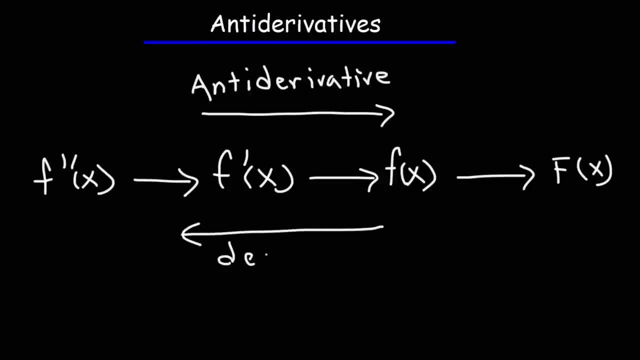 Going to the left. we're looking for the derivative. The process of finding the antiderivative is basically integration. the process of finding the derivative is differentiation. So hopefully that summarizes everything that you need to know about this conceptually. Now. we said that capital F is the integral of f, of x, dx. 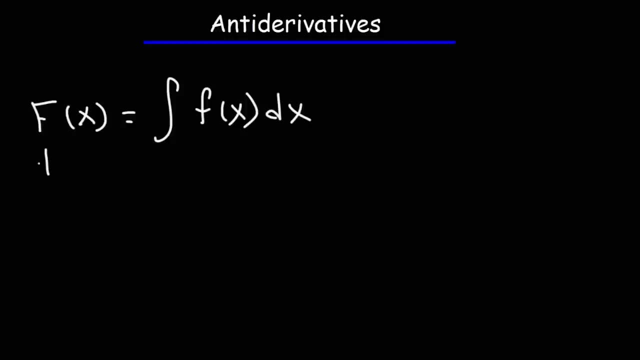 Now you get capital F plus C. You always get a constant of integration. but we're not going to worry about that here. What I'd like to do right now is distinguish what is an indefinite integral versus a definite integral. So this here is what is known as an indefinite integral. 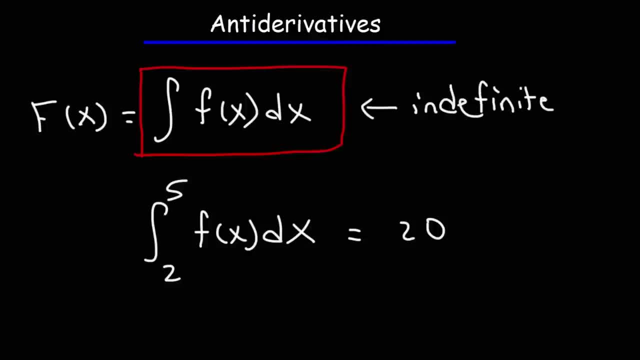 An indefinite integral. An indefinite integral gives you a function, typically in terms of x, but it could be in terms of some other variable, like y or z or something like that. A definite integral doesn't give you a function, but it gives you a number. 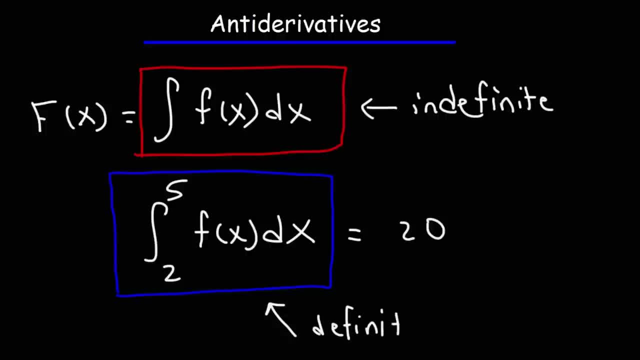 So this is a definite integral. The result of a definite integral is always a number like 20, negative 8,, 45 or something, And you can easily identify Or distinguish a definite integral from an indefinite integral. A definite integral has limits of integration. 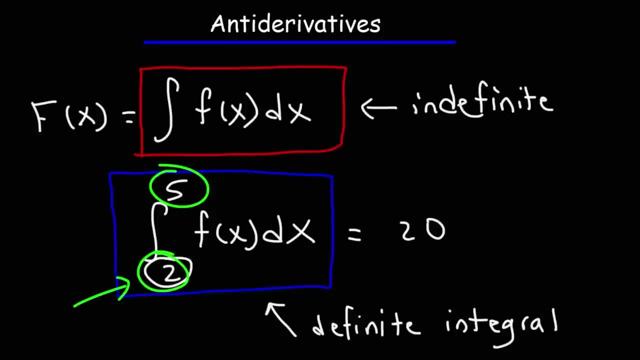 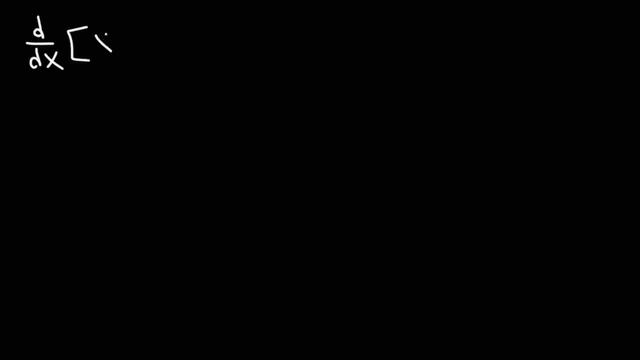 It has a lower limit and an upper limit. An indefinite integral does not have the limits of integration. So that's how you can easily distinguish between them. Now we know that the derivative of x cubed is 3x squared According to the power rule. the derivative of a variable raised to a constant is the constant times the variable raised to the constant minus 1.. 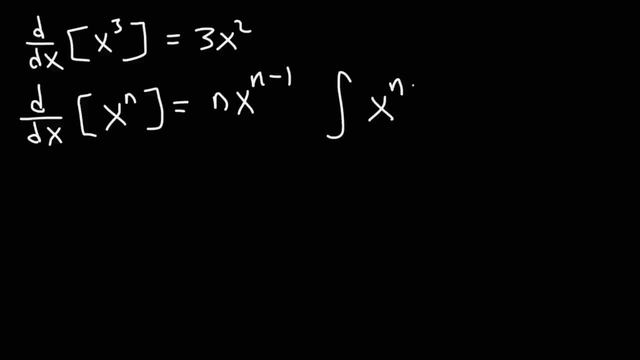 Well, the antiderivative of a variable raised to a constant is going to be that variable raised to the constant plus 1 divided by the constant plus 1.. And then plus c, the constant of integration. So that's how we could find the antiderivative of a variable raised to a constant. 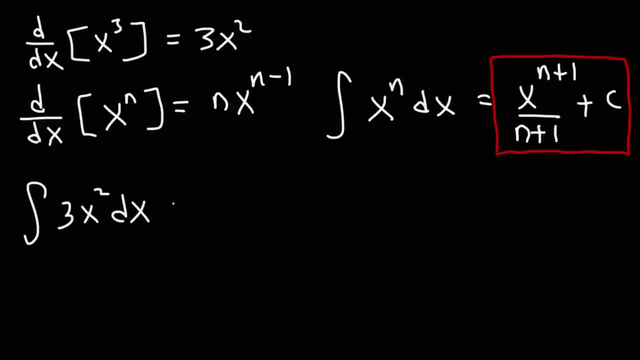 So let's find the antiderivative of 3x squared. So let's rewrite the constant Now, the variable raised to the constant that's x squared. So what we're going to do is we're going to add 1 to the exponent. 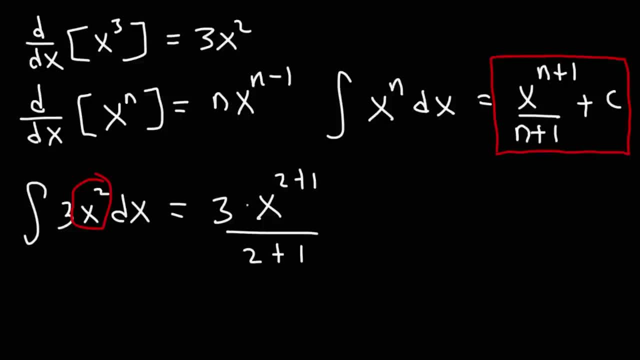 So it's going to be 2 plus 1.. And then we're going to divide it by that result, So it becomes 3x cubed divided by 3. And this gives us the original function, x cubed. But we need to add the constant of integration plus c. 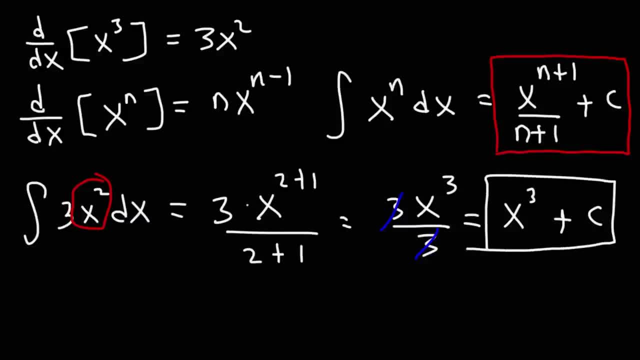 If you were to find the derivative of x cubed plus c, x cubed will become 3x squared, The derivative of a constant will become 0. So you end up with the same thing. So always when you're looking for the indefinite integral of something, 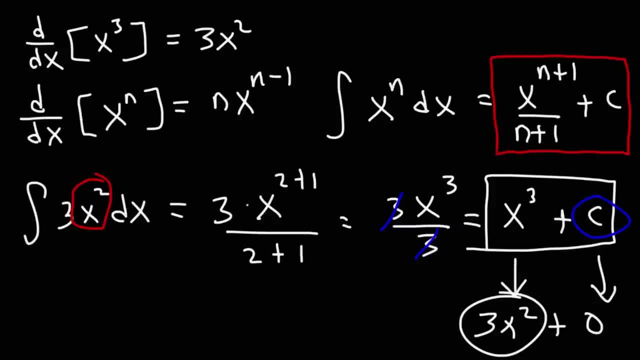 or the antiderivative, you need to put the constant of integration. The only time you don't need to worry about the constant of integration is if you're finding the definite integral where you get a number. Besides that, any time you get a function, add plus c. 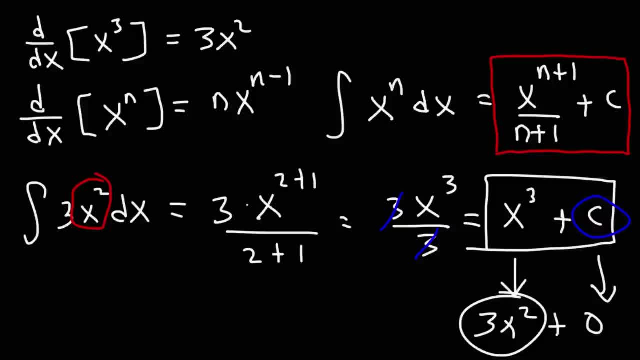 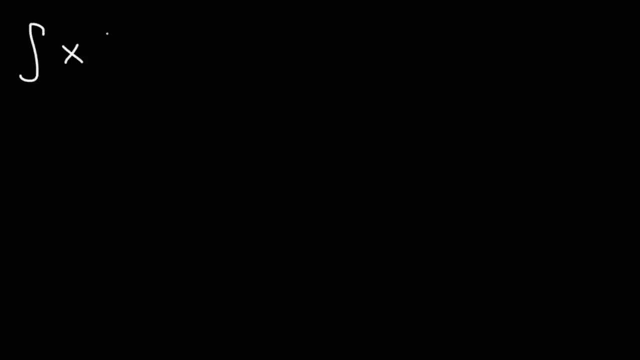 when you're looking for the indefinite integral or the antiderivative. So now let's work on some problems. Go ahead and find the antiderivative of the following functions: Feel free to pause the video and work on these examples. So for the first one, we're just going to add one to the exponent. 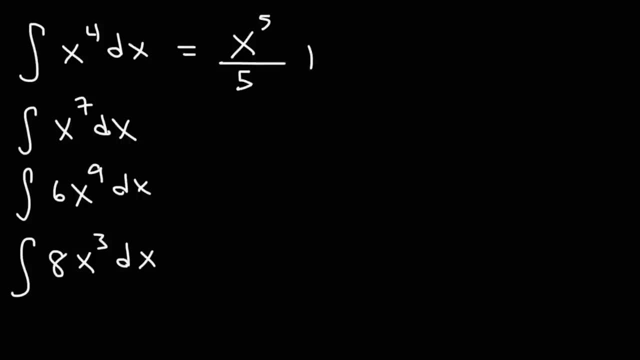 4 plus 1 is 5.. And then we're going to divide by the result And then add the constant of integration. So it's x to the fifth, power over 5 plus c. For the next one, it's going to be x to the 8 over 8 plus c. 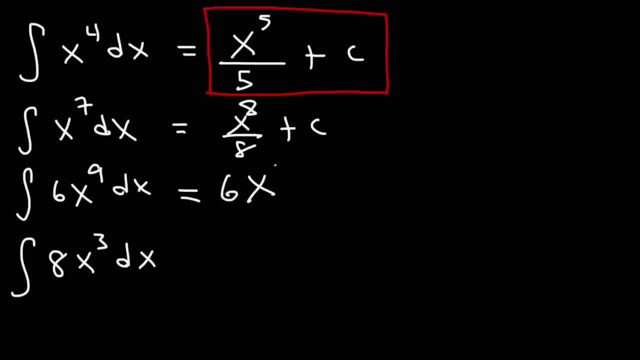 For the next one, it's going to be 6.. And then we're going to add one to 9.. That becomes 10.. Divide by 10 plus c- Now this one- we can reduce 6 over 10, if we divide both numbers by 2, that becomes 3 over 5.. 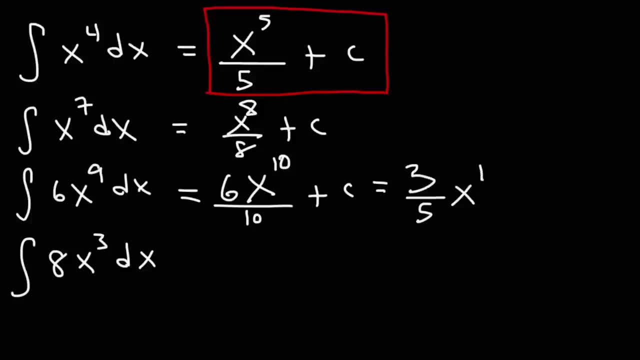 So we could say this equals 3 over 5, x to the 10 plus c. For the next one it's going to be 8, x to the 4 over 4 plus c, And we know 8 divided by 4 is 2.. 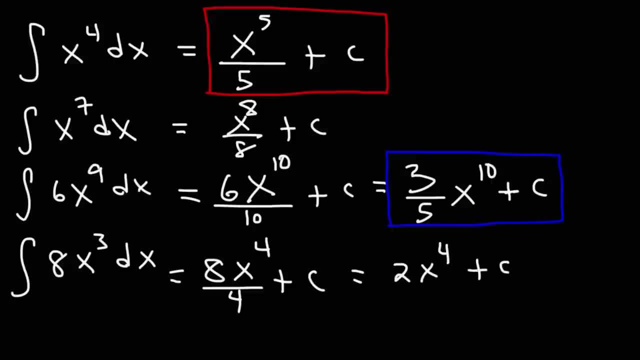 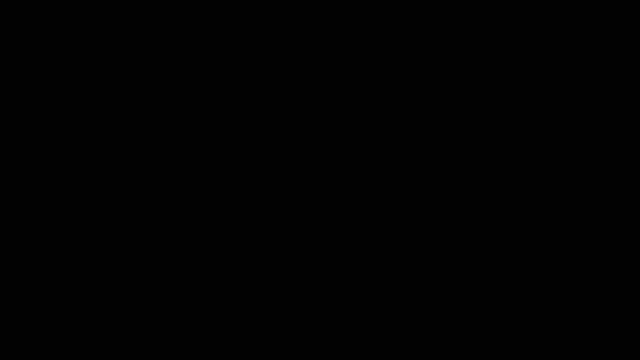 So this is 2x to the 4 plus c. So, as you can see, it's not that difficult to find the antiderivative of a function. So go ahead and try this one. Find the antiderivative of. So let's write it this way: 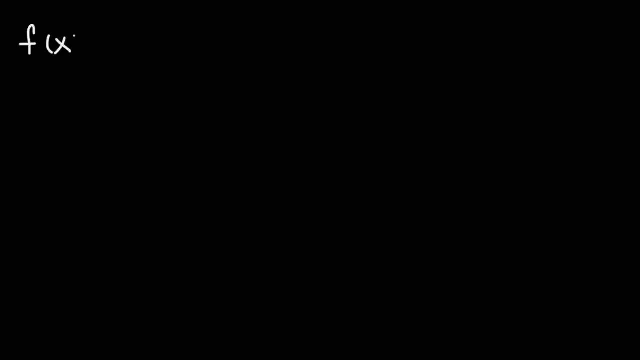 So let's write it this way. Let's say f of x is x cubed minus 4x, squared plus 8x. What is the antiderivative capital F of x of that function? So go ahead and find the antiderivative F of x. 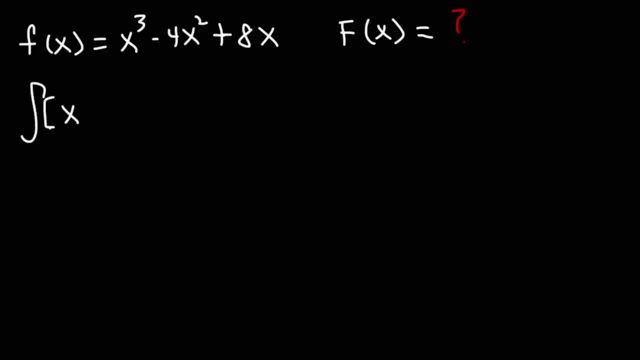 To do that, we're going to find the indefinite integral of x, cubed minus 4x, squared Plus 8x. But just to show our work, let's do it this way first. So the antiderivative is going to be the indefinite integral of f of x dx. 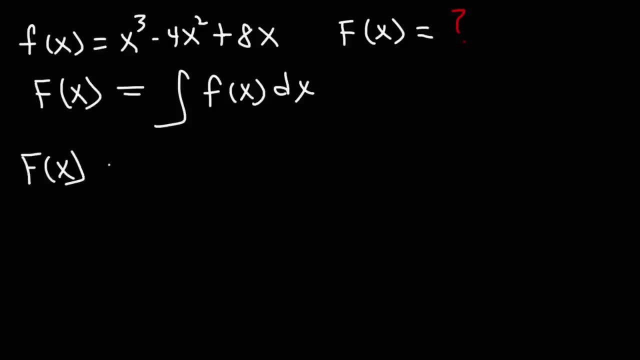 So that's the formula. And now let's replace f of x with x cubed minus 4x squared plus 8x dx. So the antiderivative of x cubed is going to be x to the 4 over 4.. 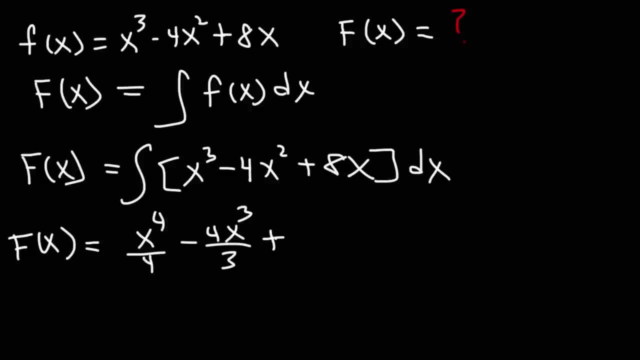 And then for 4x squared, it's going to be 4x cubed over 3.. And then for 8x, it's 8x squared over 2 plus c. Now let's rewrite it. So we're going to rewrite it as 1 fourth x to the 4 minus 4 over 3 x cubed. 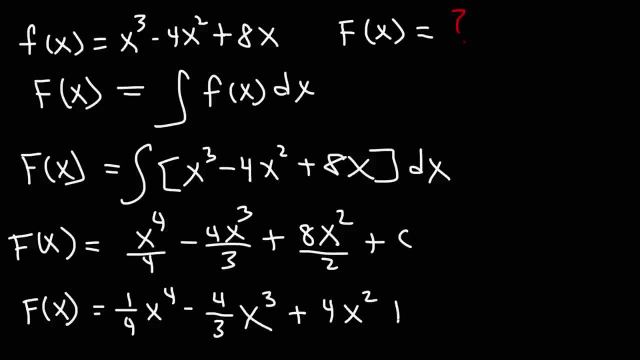 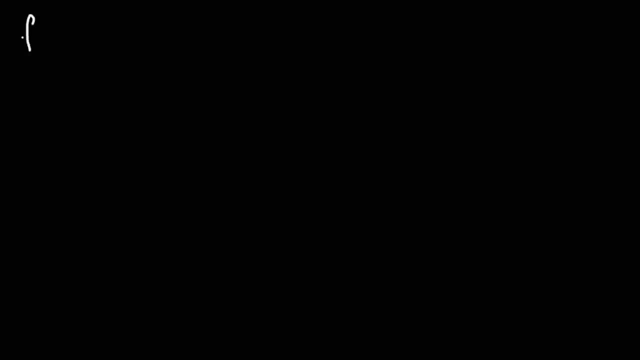 And then 8 over 2 is 4.. So we'll write that as 4x squared plus c. So this is the antiderivative of the original function. Now let's try another problem. So let's say f, prime of x. that is the first derivative of x. 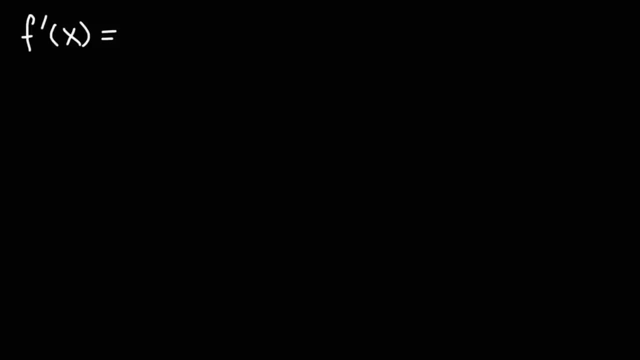 I mean the first derivative of f. rather, Let's say that's equal to 8x cubed minus 6x squared, plus 4x minus 7.. So given f prime of x, find the antiderivative f of x. 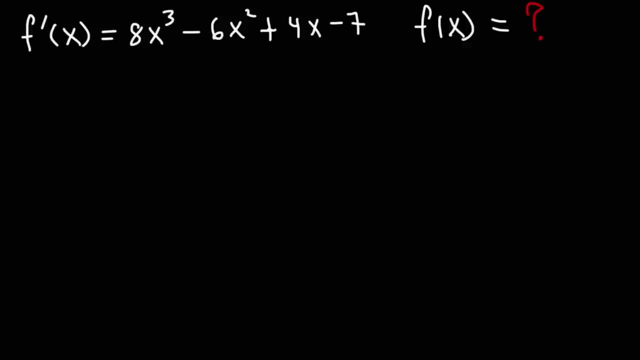 Go ahead and try that. So first let's write an expression involving indefinite integrals. We can say that f of x is the indefinite integral of f- prime of x, dx. So f of x is the antiderivative of f- prime of x. 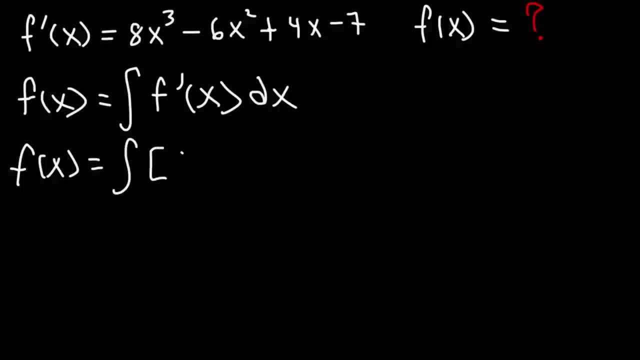 So f of x is going to be the indefinite integral of 8x cubed minus 6x, squared plus 4x, So that's equal to f of 4 x minus 7.. Feel free to pause the video if you want to try this. 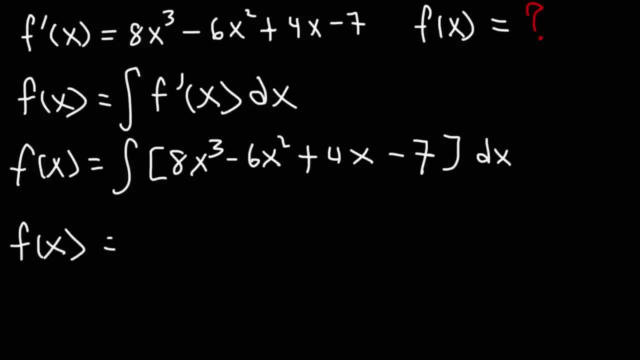 So little we can say: see you on the next lesson. And so the antiderivative of x cubed is f cubed, x to the fourth over four. For x squared, it's x cubed over 3.. The derivative of x squared is x to the fourth over 4.. 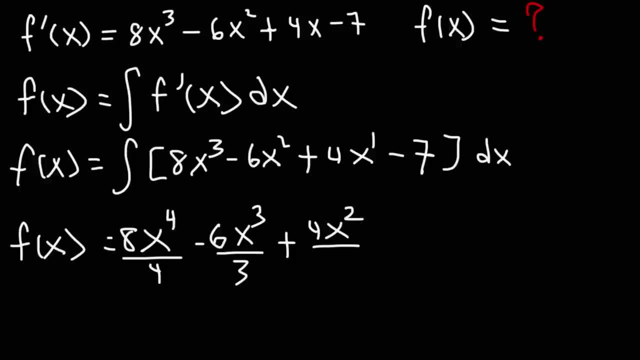 For x squared, it's x cubed over 3.. But it's a four. So the antiderivative of x cubed is x to the fourth over 4.. x to the first power, it's x squared over 2.. And then if you have a constant like 7,, 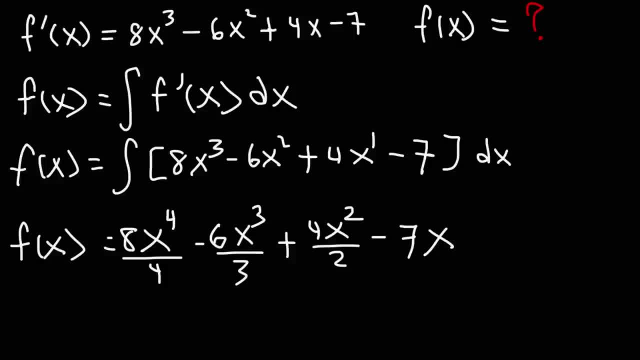 all you got to do is add an x to it. We'll talk more about that shortly- And then finally, plus c. So now let's simplify our answer. So the antiderivative is going to be: 8 divided by 4 is 2, so we have 2x to the fourth power. 6 divided by 3 is also 2.. 4 divided by 3 is: 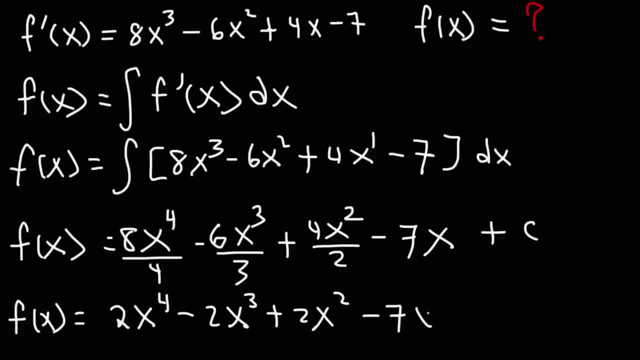 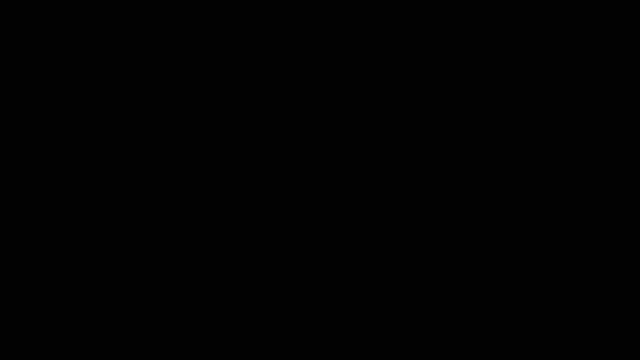 the same. So this is the antiderivative of our original function: 2x to the fourth power minus 2x cubed, plus 2x squared, minus 7x plus c. So, as you can see, it's not too difficult. 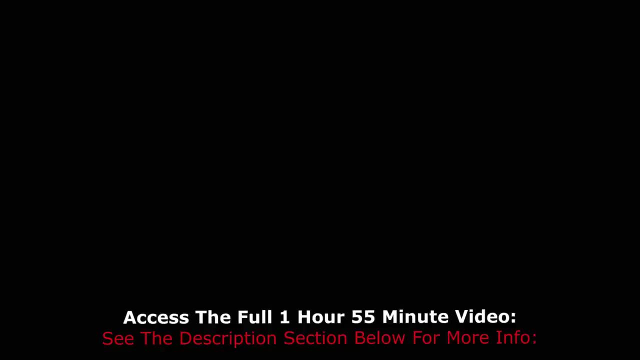 to find the antiderivative, But there are other things that you need to know. Go ahead and find the indefinite integral of d These expressions. Let's make this a, z, All right, so go ahead and try those. So let's start with the first one. We want to find the indefinite integral of a constant. 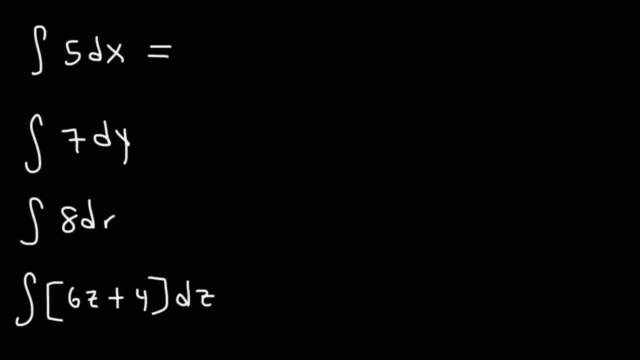 5. And we have dx in front of it. So we know it's going to be 5x, But let's see if we can get the answer using the power rule. 5 is the same as 5x to the 0. Any variable raised. 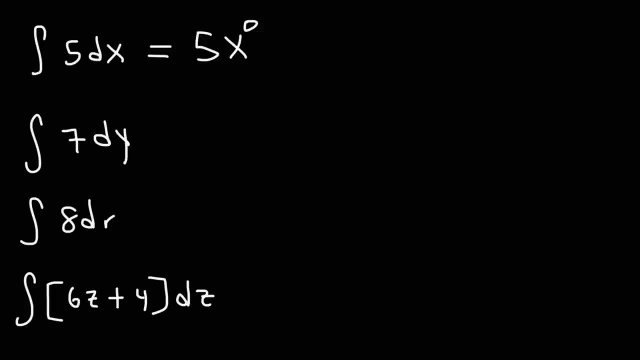 to the 0, power is 1.. So x to the 0 is 1 times 5, which is equivalent to 5.. Now, using the power rule, this is going to be 5.. We're going to add on to the exponent and then divide. 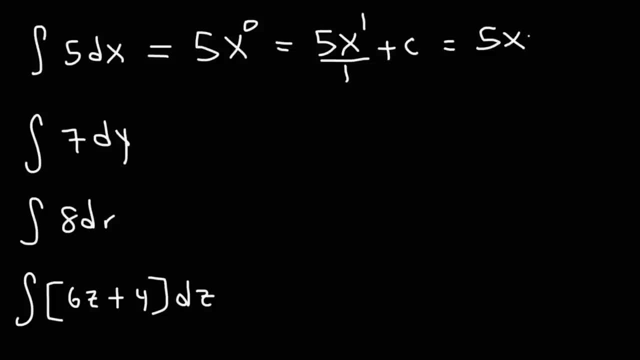 by that result. So the end result is that you get 5x plus c. So whenever you have a constant and you wish to integrate that constant, just add a variable to it. Now, the variable that you should add is based on what you see here: Either dx, dy, dr or dz. 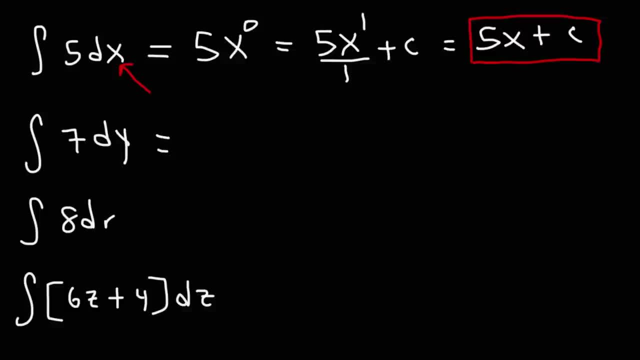 So what is the end result? This is the indefinite integral of 7dy. So instead of 7x, this is going to be 7 times y plus c. So the differential dx- dy. it tells us what variable we should be adding to the constants. 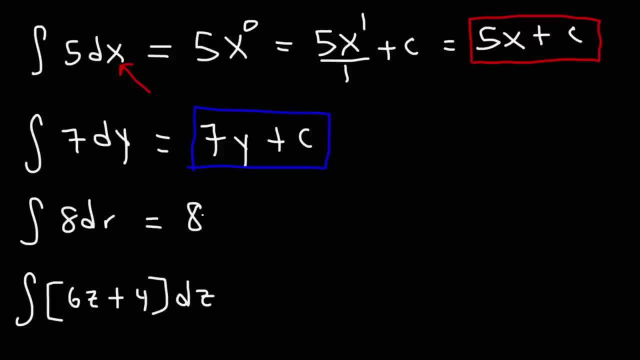 The indefinite integral of 8dr. that's going to be 8 times r plus c. For 6z plus 4, it's going to be 6.. And then z to the first power. that becomes z squared over 2.. 4 becomes 4z, and then we'll add: 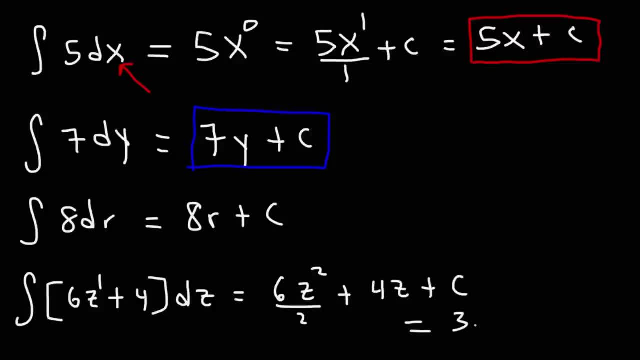 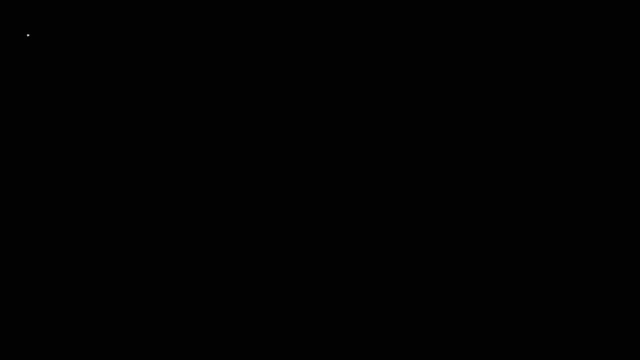 plus c. So this we could simplify it as 3z squared plus 4z plus c, So that is the indefinite integral of 6z plus 4.. Try this problem. So let's say you're given the first derivative of f And let's say it's 7.. This should be not f of x but f prime of y. So let's say it's 7y cubed. 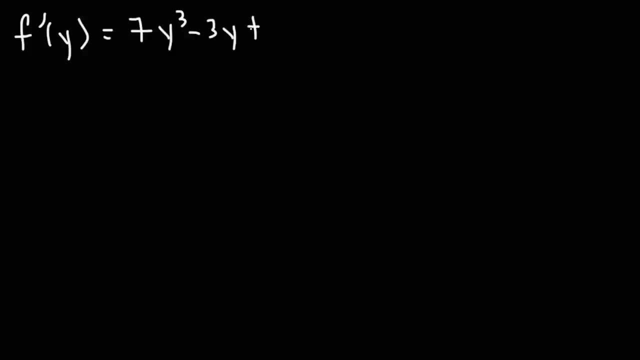 minus 3y plus 8.. And your goal is to find capital F of y. How would you do it? Feel free to pause the video and try it. So first let's write a mental outline of what we need to do here. We're given the first derivative. 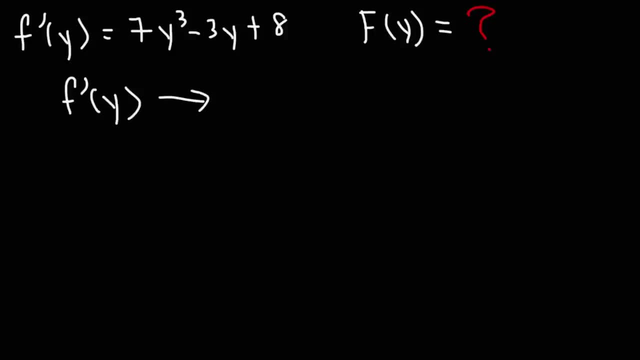 of f. We need to find f. So f is the antiderivative of f prime. but we're not going to stop there. We need to find capital F. So what we need to do is we need to integrate the function two times. 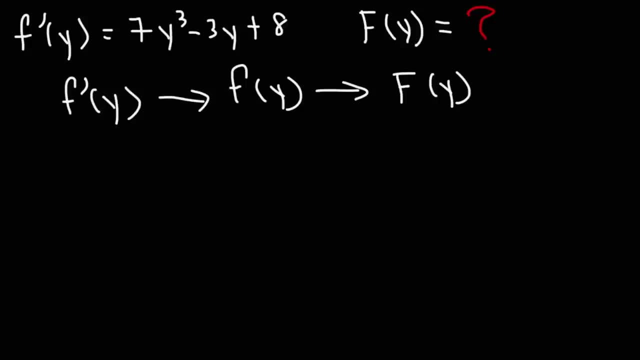 So we have a successive integration problem. So first let's integrate it the first time. Let's find regular f or little f. So this is going to be the indefinite integral of f, prime of y, dy. So that is the indefinite integral of 7y cubed minus 3y. 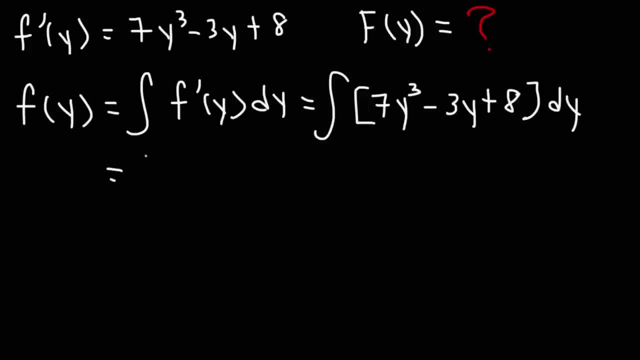 plus 8.. So the antiderivative of y to the third is going to be y to the fourth over 4.. The antiderivative of y is y squared over 2. And for the constant 8, it's just going to be 8y, based on what we have here: dy And then plus the constant c. 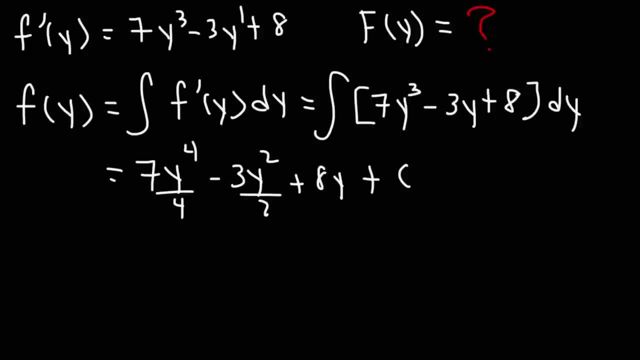 So that's f of y. We don't know what the value of c is. If we were given a point of f of y, we could find c, but we'll save that for another problem. So this here is the general function of f of y. 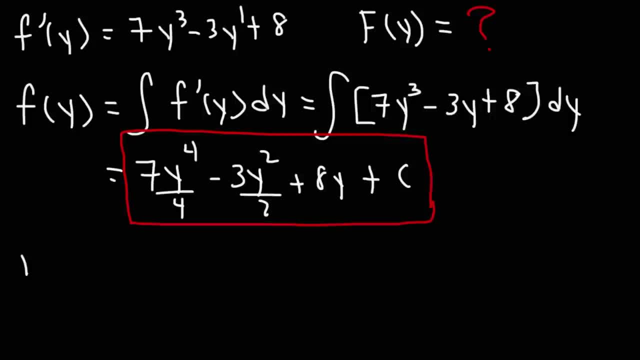 So now let's find capital F of y. That's going to be the indefinite integral of f of y, dy. So that is the indefinite integral of 7 over 4, y to the fourth, minus 3 over 2, y squared plus 8y. 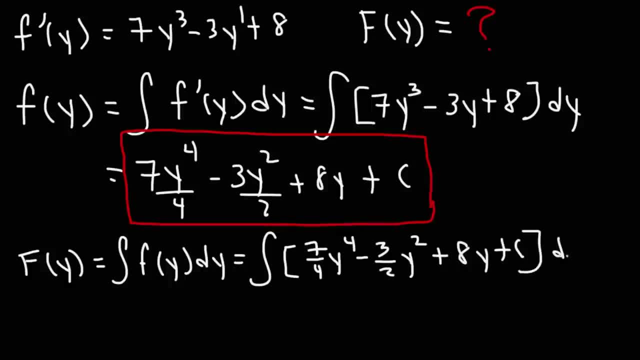 Plus c as well, And we're going to have dy. So the antiderivative of this, we're going to rewrite the constant and then we'll find the antiderivative of f of y. So that's going to be y to the fifth over 5, and then minus. 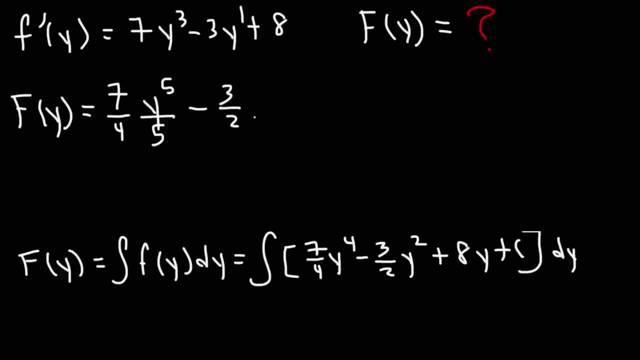 Let's rewrite the constant first, So we have 3 over 2, and then the antiderivative of y squared is going to be y to the third over 3. And then it's going to be plus 8 times y squared over 2.. 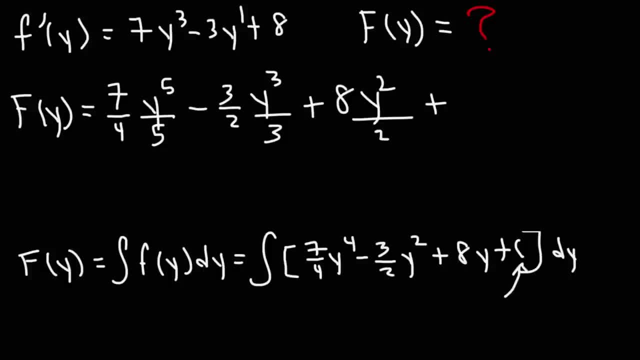 Now we have the constant of integration, c, So we're going to add a y to it. It's going to be c times y, and then plus a new constant which we'll call d, So this becomes 7 over 20, y to the fifth. 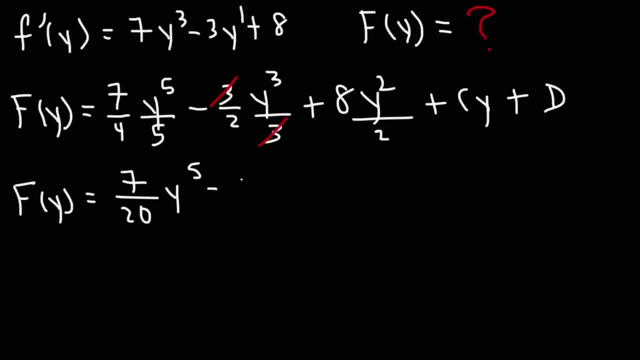 Here we can cancel the threes. So it's going to be minus 1 half y to the third plus 4, y squared plus cy plus d, So that is the second antiderivative of f, prime of y, which is capital F of y. 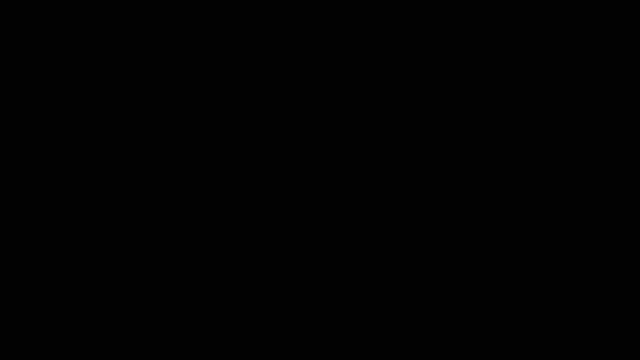 By the way, for those of you who want access to the full length version of this video, check out the links in the description section below. If you join my YouTube channel membership program, you can get access not only to the full length version of this video, but many other full length versions of this video. 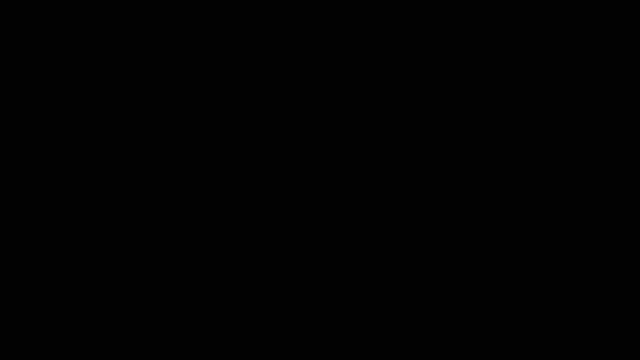 You can also check out the full length version of other videos that I have on YouTube, which you'll see over time, So feel free to take a look at that when you get a chance. Now let's work on finding the indefinite integral of other types of functions. 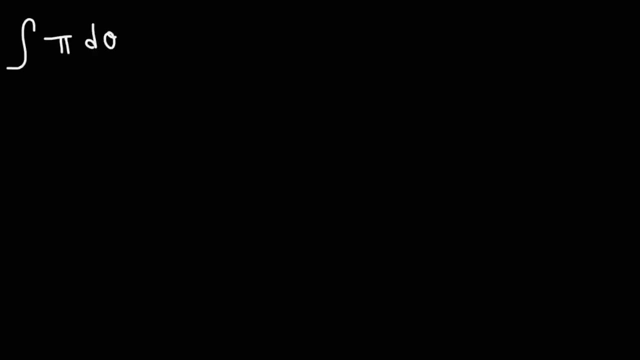 What is the indefinite integral of pi d theta? Feel free to pause the video and work on that. And what is the indefinite integral of e? let's say e ds. So pi is a constant. Let's compare it to the indefinite integral of 7 dy. 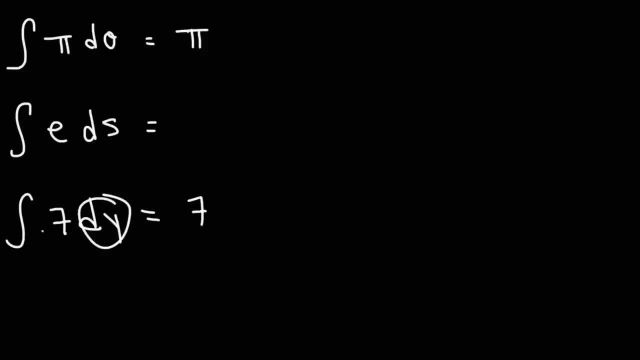 7 is a constant and we would add the variable y to it, so this will be 7y plus c. So pi is a constant And here we're going to add the variable theta to it plus c. So that's the indefinite integral of pi d theta. 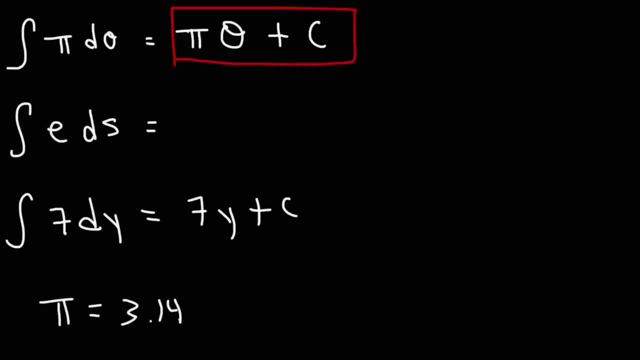 So remember pi is a constant. It's 3.14 with some other numbers. after that Let me find out what those other numbers are. So it's 3.141592654 with some other numbers. So whenever you see pi, it's just a constant. 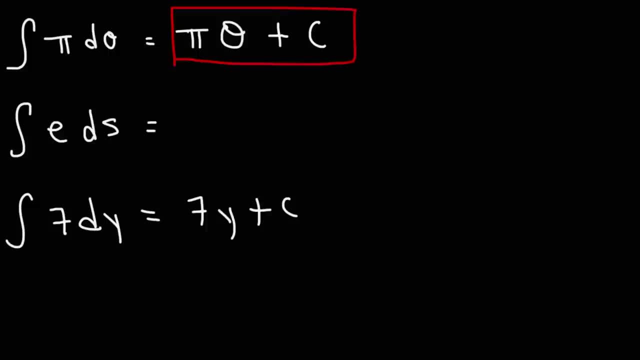 So treat it as if it's any other number, like 7 or 8 or negative 4.. The same is true for e. e is not a variable, it's a constant. e is equal to 2.71828, and so forth. 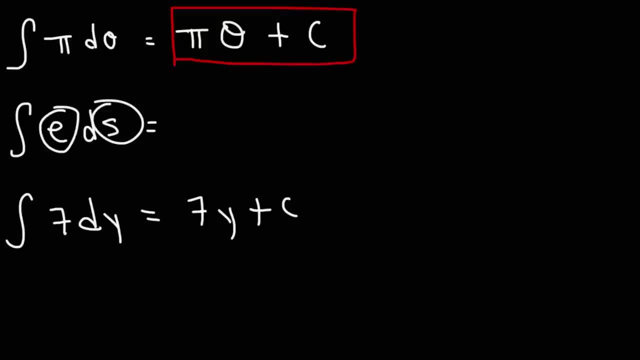 So, when looking at a problem like this, e is the constant, s is the variable, So this is going to be e times s plus c. Whenever you're finding the indefinite integral of something, you need to be able to distinguish the constant from the variable. 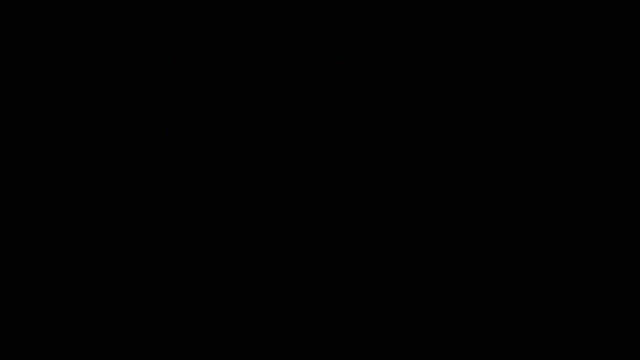 in order to integrate it properly. Now let's focus on finding the indefinite integral of rational functions. What is the indefinite integral of 1 over x squared? To find this, before you integrate it, you need to rewrite the expression. We need to move the variable from the bottom to the top. 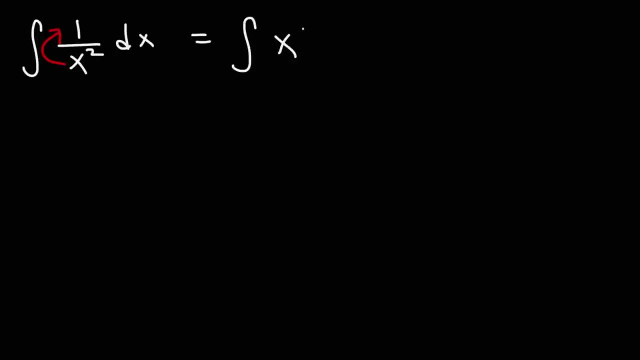 So this is x to the negative 2.. At this point we could use the power rule So we can integrate it by adding 1 to the exponent. So it's going to be negative 2 plus 1 and then dividing by that result plus c. 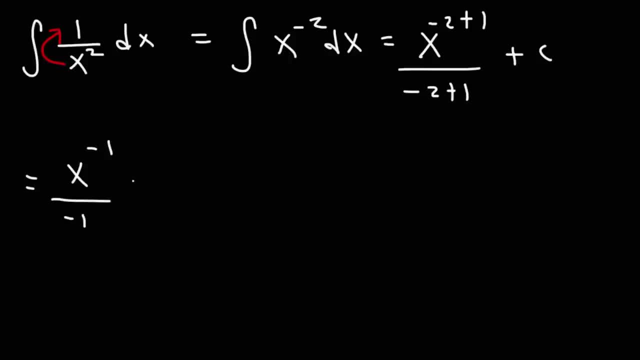 Negative: 2 plus 1, that's negative 1.. And after you integrate it you need to rewrite it again. So we want to get rid of this negative exponent. So we can do something. So by moving the variable back to the bottom. 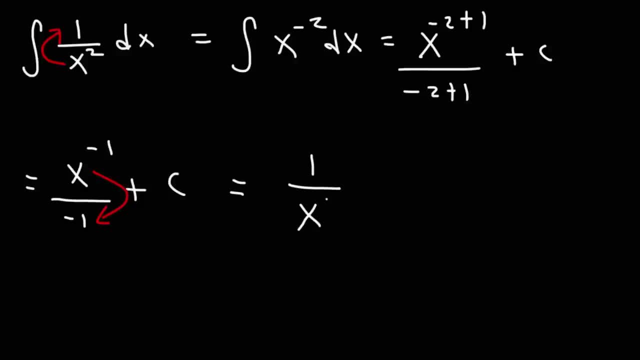 So that leaves a 1 on top. And then we're going to have x to the first power on the bottom, which we can just leave as x, The negative sign. I'm going to move it to the top. So the final answer is negative: 1 over x plus c. 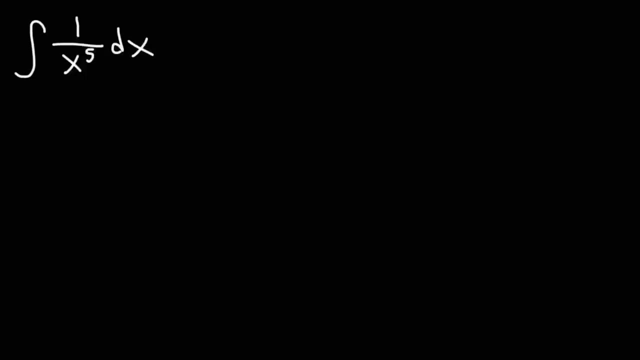 Now let's try this one. What is the indefinite integral of 1 over x squared? So we have an integral of 1 over x to the fifth power, dx. So feel free to pause the video and try it. So, just like before, let's move the variable to the top. 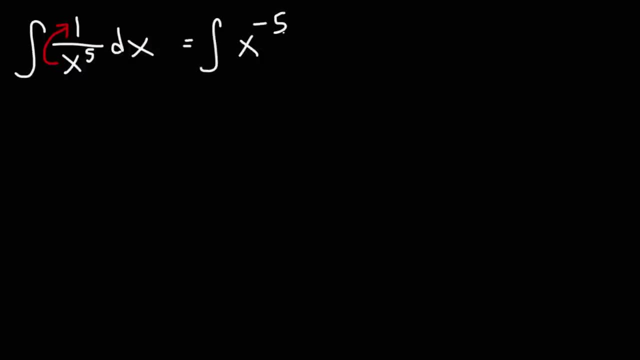 So we have the integral of x raised to the negative 5, dx, And then let's add 1 to that. So negative 5 plus 1 is negative 4. And then we're going to divide by that result. Next let's rewrite the expression. 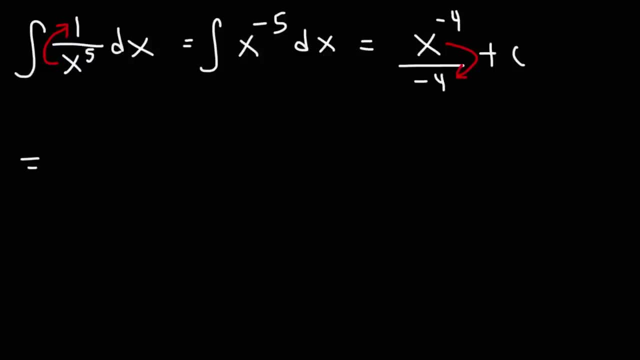 So we're going to move the variable back to the bottom And the negative sign we're going to move it to the top. So we're going to have negative 1. We have a 4 on the bottom and x, And then this negative 4 becomes positive: 4 plus c. 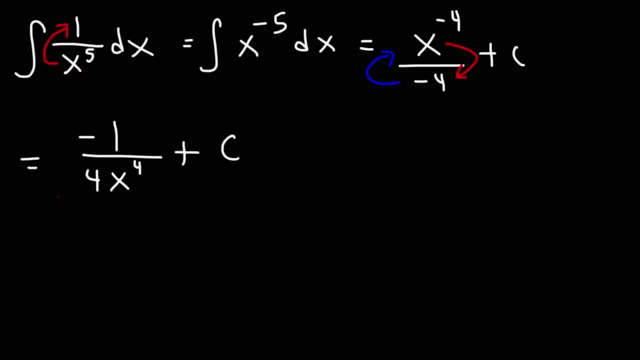 So negative 1 over 4x to the fourth plus c, That is the indefinite integral of 1 over x to the fifth power. Try this: Find the indefinite integral of 7 over x, cubed dx. So, like before, we're going to move the variable to the top. 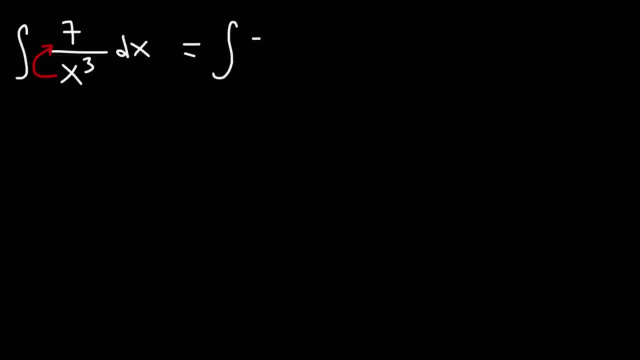 So we're going to rewrite the integral. So this is 7x to the negative 3,, dx. And now let's integrate: So negative 3 plus 1, that's negative 2.. And then we're going to divide by negative 2.. 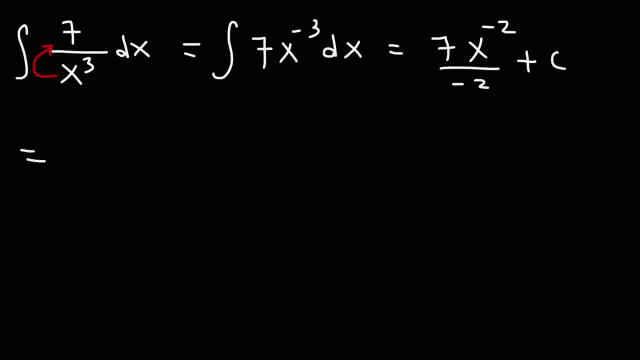 And then we'll have plus c. So next we're going to move the variable back to the bottom And the negative sign I'm going to move to the top. So this becomes negative 7.. We have a 2 on the bottom. 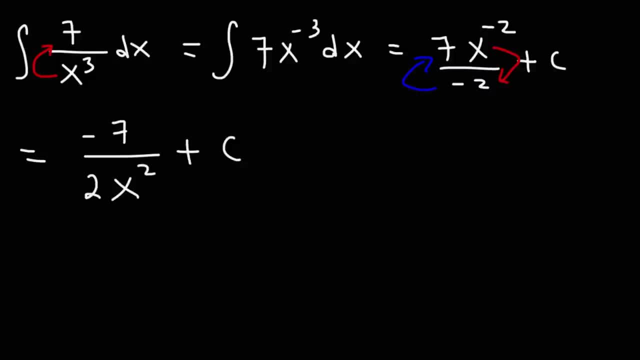 And we have x squared as well. So it's negative 7 over 2x squared plus c. So that's how you can integrate rational functions. Go ahead and try this expression: Find the indefinite integral of 5x to the 7 minus 9 over x squared plus 4x minus 8, dx. 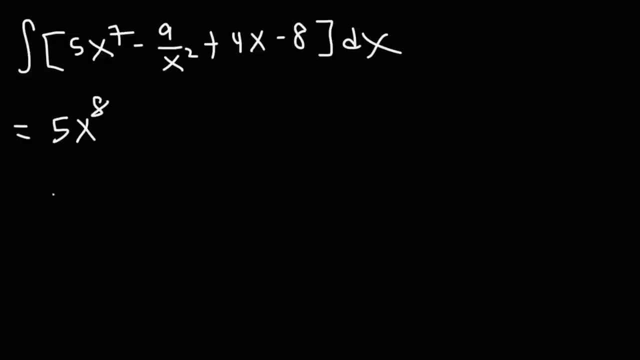 So this is going to be 5x to the 8 over 8.. Now for negative 9x squared. we need to write that as negative 9x to the negative 2.. So that's going to be negative 9x. negative 2 plus 1 is negative 1, divided by negative 1.. 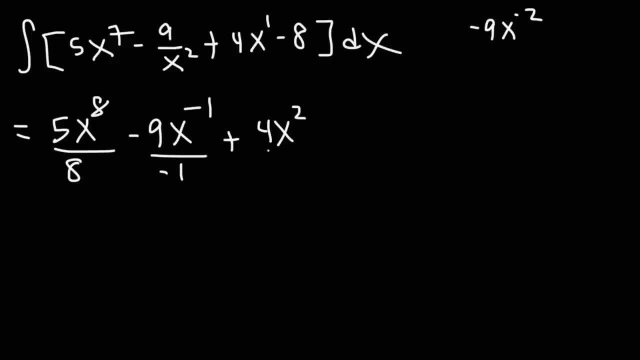 And then for 4x to the first power, that will be 4x squared over 2, and then minus 8x plus c, So we can rewrite this as 5 over 8, x to the 8, plus 9.. 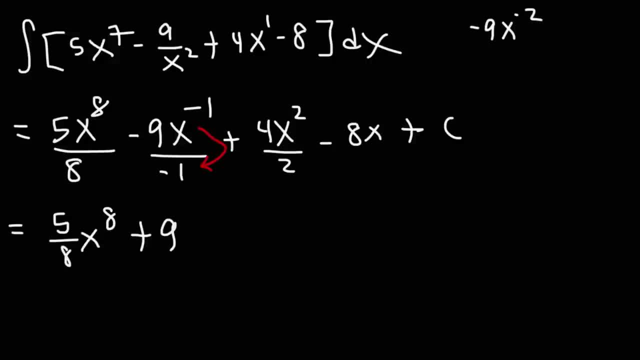 The two negative signs will cancel and then we can move the x variable to the bottom. So it's plus 9 over x and then plus 2x squared minus 8x plus c. So that is the indefinite integral or the antiderivative of this expression. 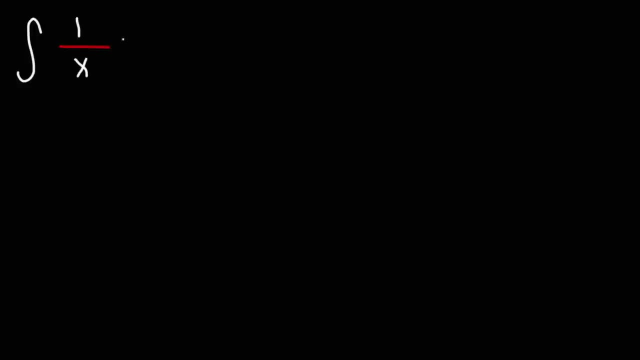 Now, what is the antiderivative? The antiderivative of 1 over x, dx. What do you think we need to do here? Well, if we were to try the same approach that we've been using for rational functions, let's say, if we were to rewrite the expression by moving x to the top. 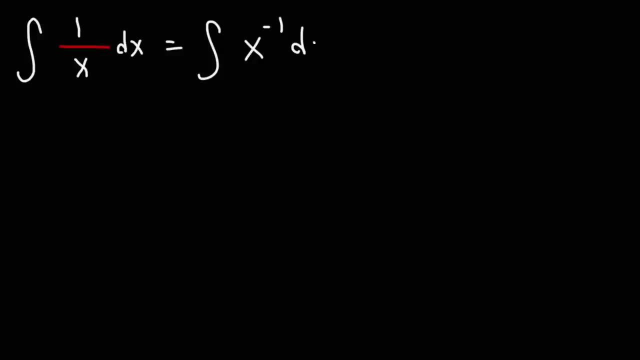 we would get the indefinite integral of x to the negative 1, dx. Now, using the power rule, if we add 1 to negative 1, we'll get x to the 0. And if we were to divide by that result, 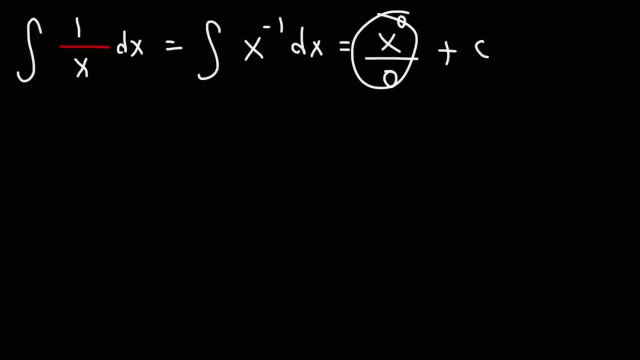 we would get something that is undefined, So this technique doesn't work for 1 over x. Instead, this is an integral that you should commit to memory. The integral of 1 over x- dx is simply ln x, So you may want to add that to your list of notes. 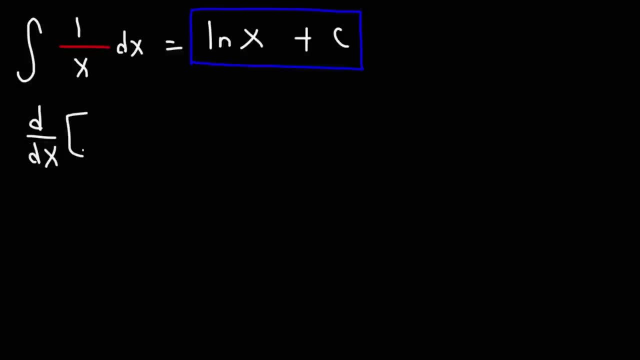 And if you recall, the derivative of ln- u, where u is a function of x, is u prime over u. So the derivative of ln x is going to be u prime. If u is x u prime, the derivative of x is 1.. 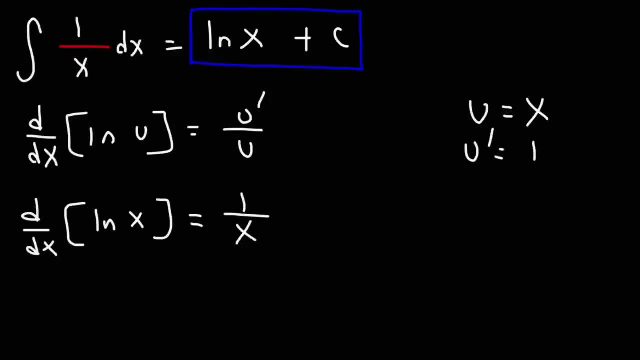 So we get 1 over x. So that's the antiderivative of 1 over x to the first power. So if the antiderivative of 1 over x is ln x, what is the antiderivative of 1 over x plus 3?? 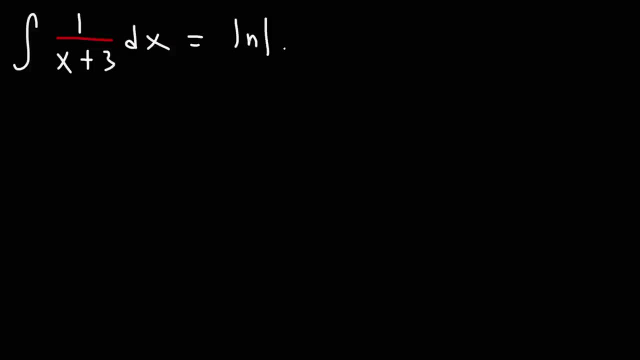 This is simply the natural log of x plus 3.. So, based on that, go ahead and find the antiderivative of the following: One over x minus 5, dx, 5 over x plus 2, dx And 7 over x plus 4, dx. 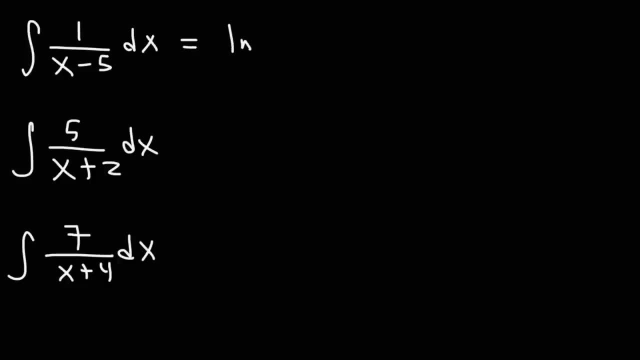 So this is going to be the natural log of x minus 5 plus c. Now, typically, if your answer is like different than ln, x, normally you'll see an absolute value around x minus 5.. And the reason for this is that you can have a negative number. 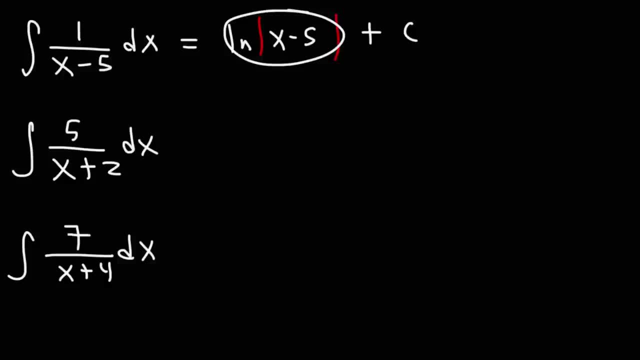 inside the natural log. It's going to be like it's going to give you an error in the calculator, So typically you'll see an absolute value symbol for expressions that can be negative. For the next one, let's move the constant to the front. 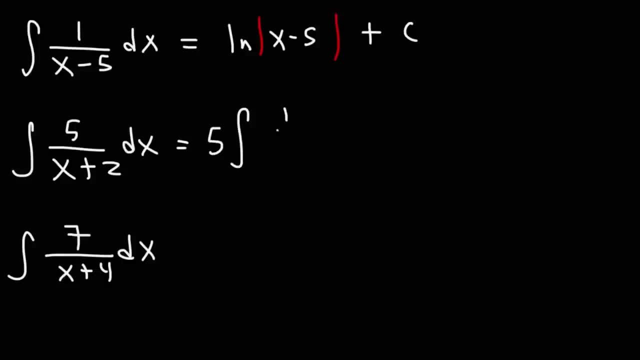 So think of this as 5 times the integral of 1 over x plus 2, dx. So this is going to be 5 times the natural log And let's put our absolute value symbol. So it's 5 ln. x plus 2, plus the constant of integration. 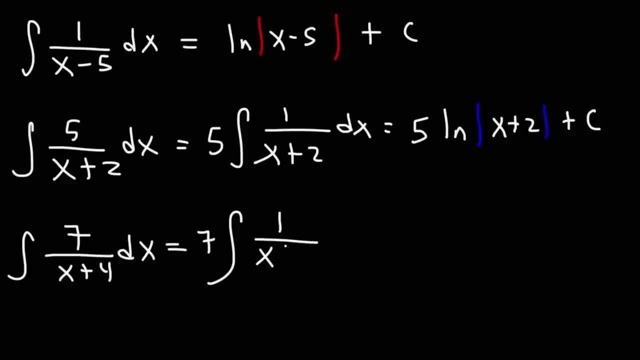 For the next one, let's do the same thing. Let's move the constant to the front, So this is going to be 7 ln, x plus 4, and then plus c. So that's how you can integrate rational functions where the denominator is a linear function. 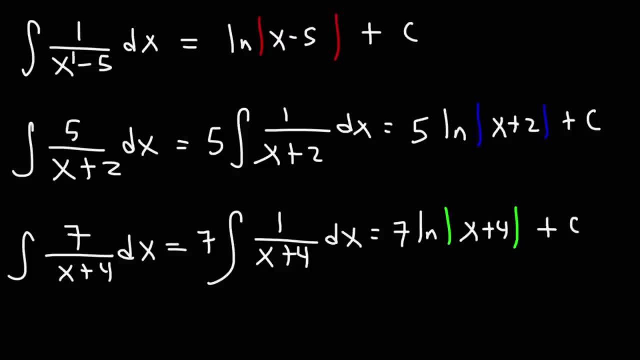 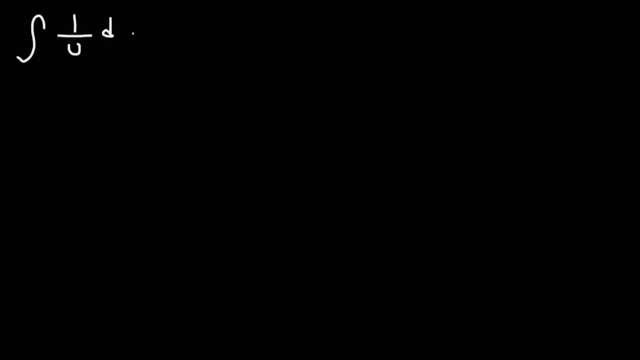 like x plus 2,, x minus 5, and so forth. Now here's a general formula That you can use when integrating rational functions like 1 over u. where u is a function of x, It's going to be 1 over u prime. 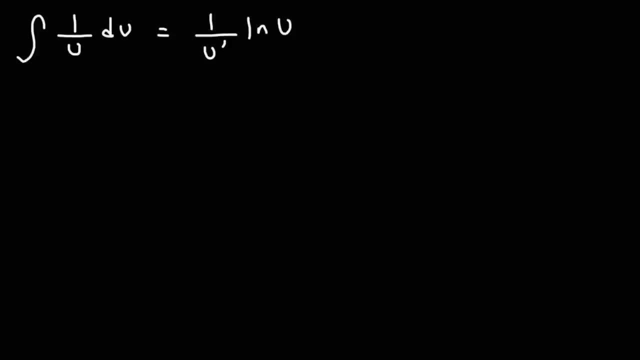 times the natural log of u plus c. Now this works if- and this is a big if- if u is a linear function in the form ax plus b, Now a could be 0, b could be 0. Well, if a is 0, it doesn't work, but b could be 0. 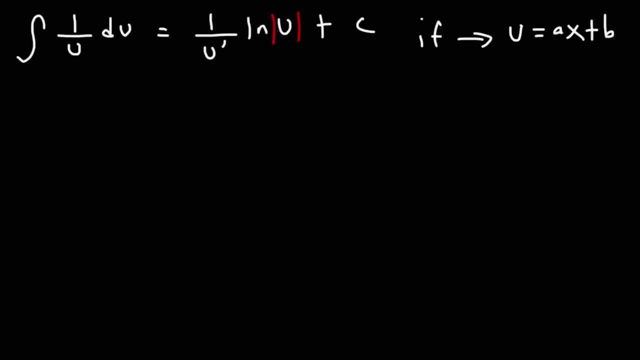 But u has to be a linear function. in that form, If there's like an x squared or an x cubed, this formula is not going to work. So let me repeat that u has to be a linear function If you have a square root of x. 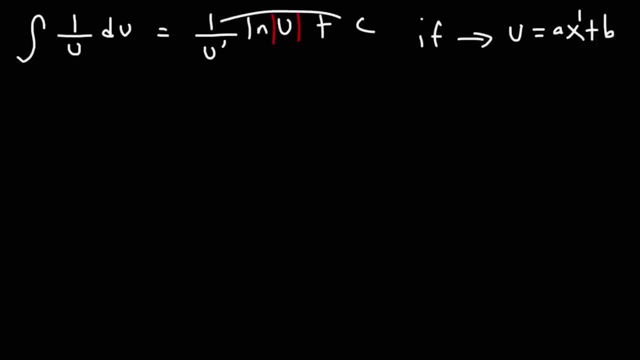 or anything but x to the first power. this will not work. So now let's try some harder examples. Based on that, what is the indefinite integral of 1 over 3x plus 4?? And let's compare that to the indefinite integral. 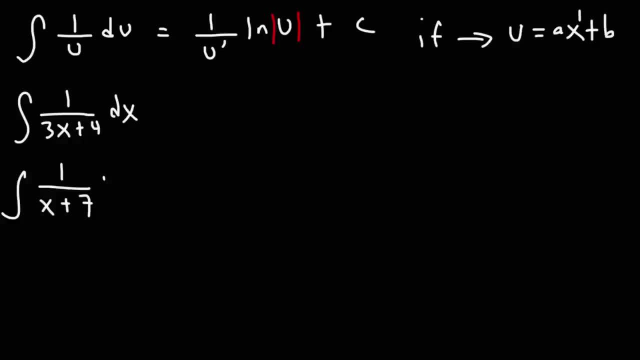 of 1 over x plus 7.. So in this case we can see that u is 3x plus 4.. The derivative of u, which is u prime, the derivative of 3x, is 3.. The derivative of 4 is just nothing. 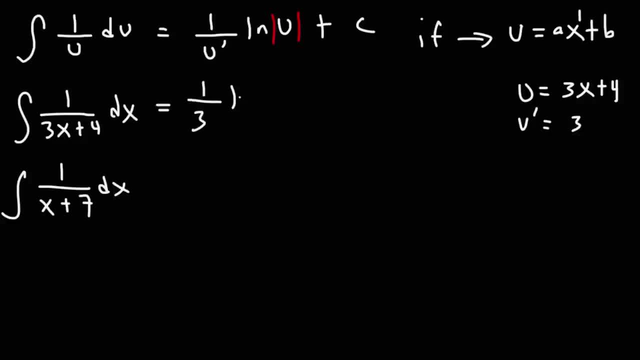 So u prime is 3.. So this becomes 1 over 3 ln, absolute value, 3x plus 4, and then plus c. So this fraction is a result of the derivative of that expression. For the next one, the derivative of x plus 7, is just 1..